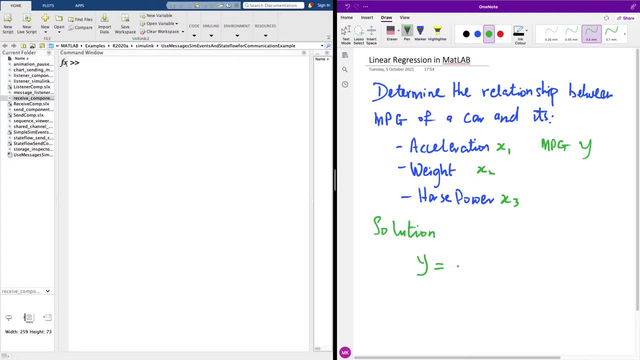 so basically we have a model like this: y is equal to beta 0 plus beta 1 x 1, plus beta 2 x 2 plus beta 3 x 3.. So I want to determine this coefficient so that we can actually plug it into. 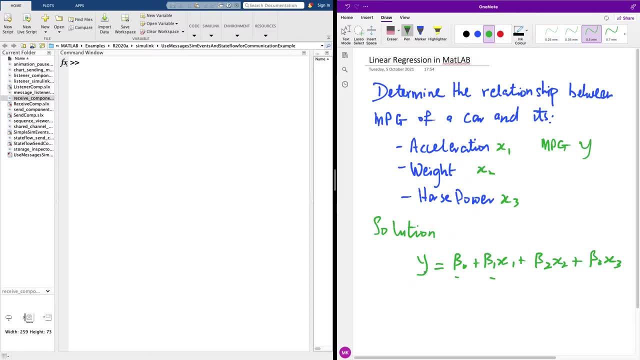 this equation to determine now the function that relates the mpg, which is y, and the values of x1, x2 and x3, which is acceleration weight and the horsepower. So let me quickly use MATLAB to show you how to solve it. So the data set we are going to be using is called the K-small data set. 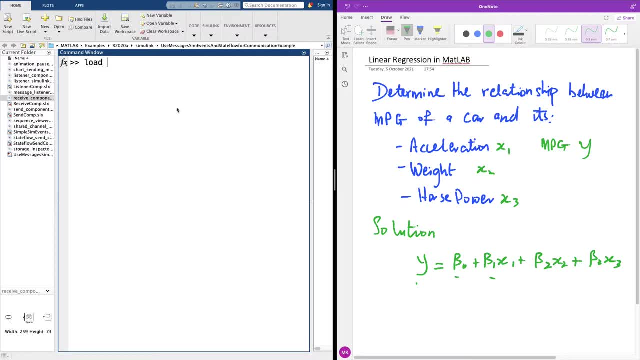 So if I is a free data set available in MATLAB, so if I say load car small, so it looks of this data safe and you can see, at this point we can see the features of this data set: the acceleration, the cylinder, the displacement and the mpg and so on, but we don't know this. 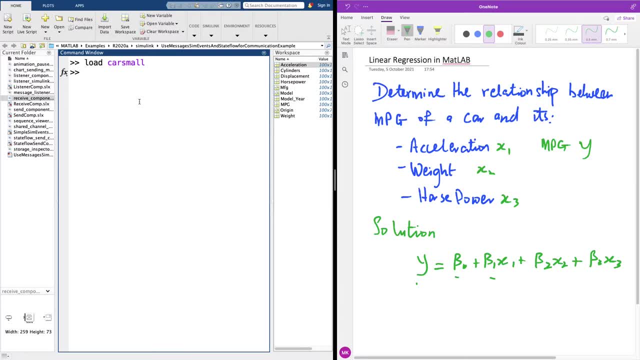 relationship. and now I want to use linear regression- linear, multiple linear regression- to solve it. Now, if you want to see these variables individually, you can just type them. for instance, you want to see cylinder- cylinder- as you can see value for cylinder- and to play the screen, I can just use clc. 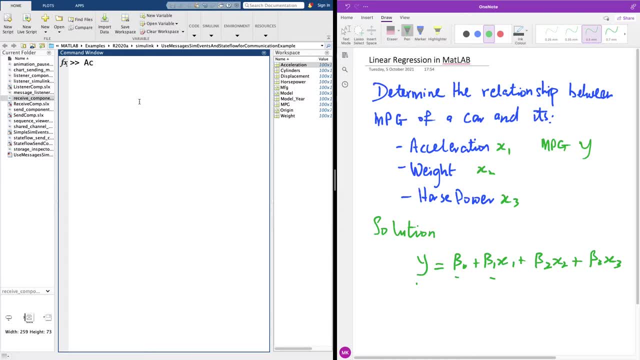 and if you want to see the acceleration, you can just type it as well- acceleration- and you can see the oh sorry, so this is going to be acceleration, yeah, like this, and so on. All right, so you can take take some time to look at this data set and see what you can make from it. 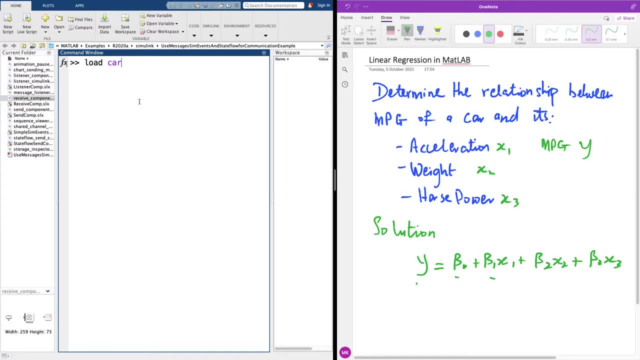 Let me look back my data set. loads car small, All right, so to do linear regression. the first thing we want to do is we want to extract the values, I mean the columns we want to use. because you don't want to use all the columns, the instructions say you want to use only these three columns: one, two, three and here. 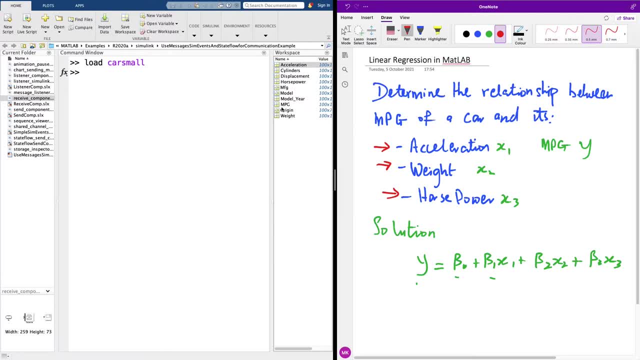 you have, we here, we have so many columns here. so first of all, extract these columns, these three columns in the column, into a variable x. So I'm going to say x is equal to, let's see, acceleration, and weight and horsepower is like this. All right, So I want to extract these variables first into an array like this: Okay, So if I look at the value of x, you can see that we now have the values, the data set for x. Okay, 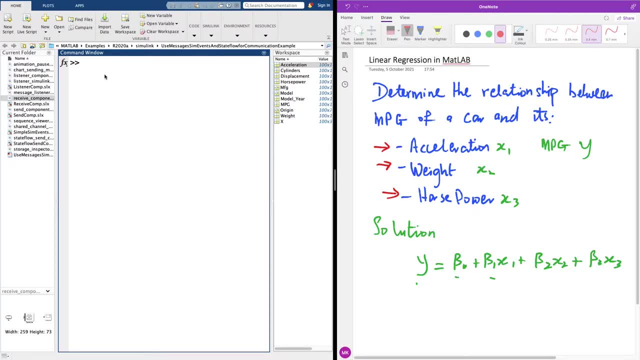 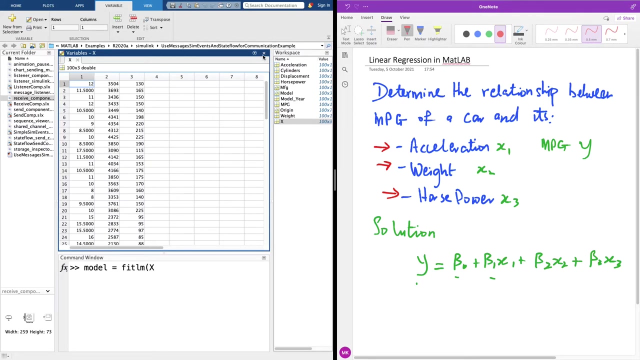 All right. So the next thing I would like to do is to create a linear model- Let me call it model is equal to model is equal to fit linear model- and specify the x data set we already have, because you can look at the x data set right here in this data frame by simply double clicking on it. So I'm going to go back to Charlie. I can keep this open or I can actually close it. 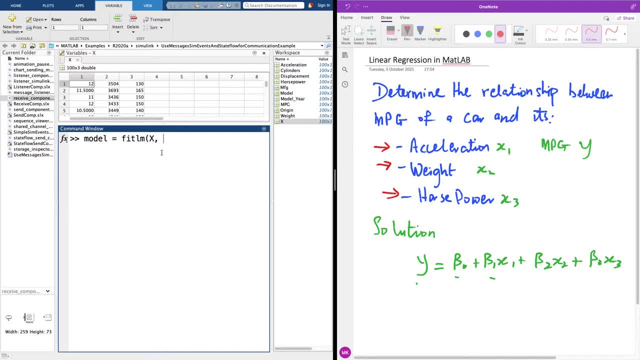 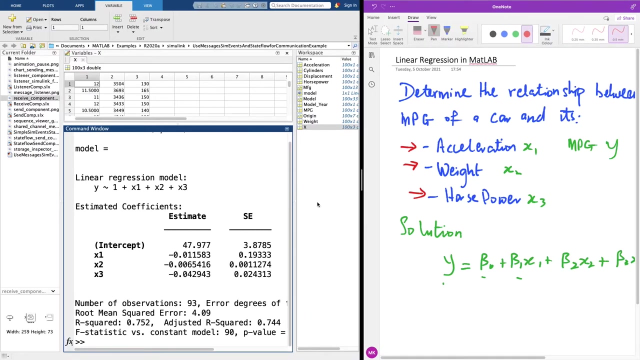 All right, So specify x and specify the y value. In this case we have it is mpg. So I want to fit a model between the x data set here and the mpg to find some relationship, And I'll simply hit the enter key. Now, if you hit the enter key at this point, it's going to provide you all the metrics that is needed. Now we are not interested in all these metrics, We're only interested for now, to keep it simple. 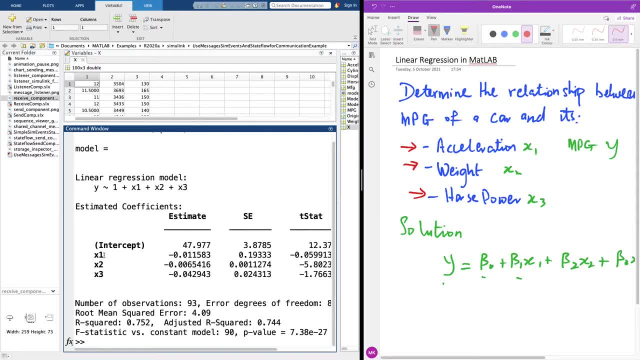 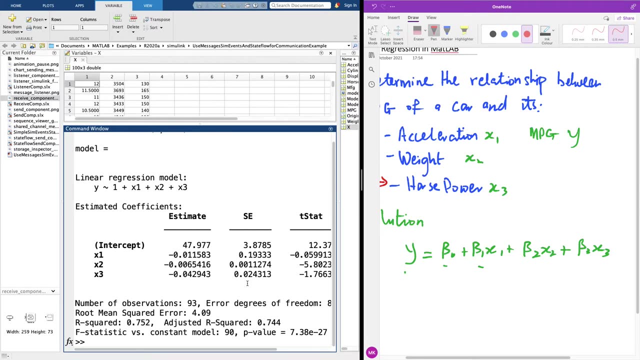 We are interested in the intercept. So this intercept is x1, x2, and x3.. Okay, So at this point you can actually plug in the intercepts for the value for y and get the values for x. So this is basically how to solve a linear regression in MATLAB. So you have the values for the estimate for x3.. You have the intercept and you have the x1, x2.. 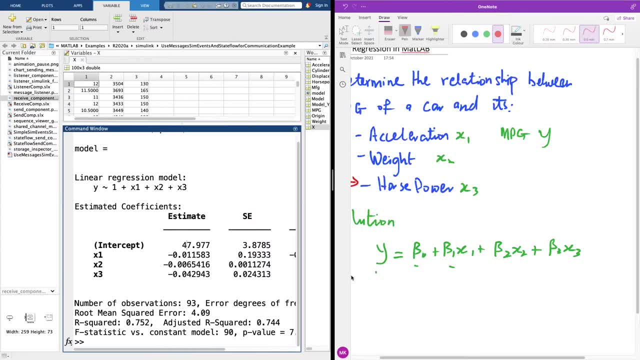 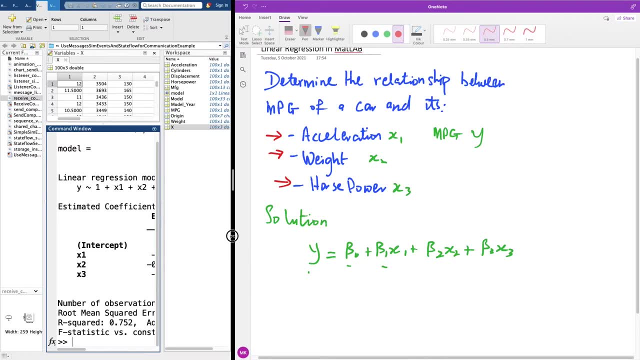 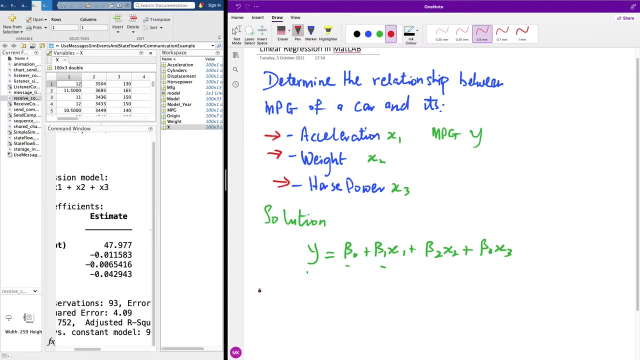 So I can actually write out this equation literally at this point. So permit me to kind of make some room here, And then you can just shift this away a little bit and just shift this one, So I can now write the equation to be y or mpg. Sorry, let me just use y as a function of x, So I can say y is equal to beta, 0 is 47.. 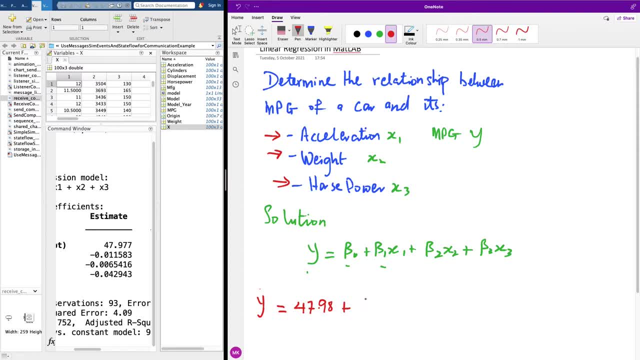 98 plus. beta 1 is, in this case, is going to be a minus. So let me just take out this and use a minus. So it's going to be minus. beta 1 is 0.0115 x1.. So it's going to be x1.. 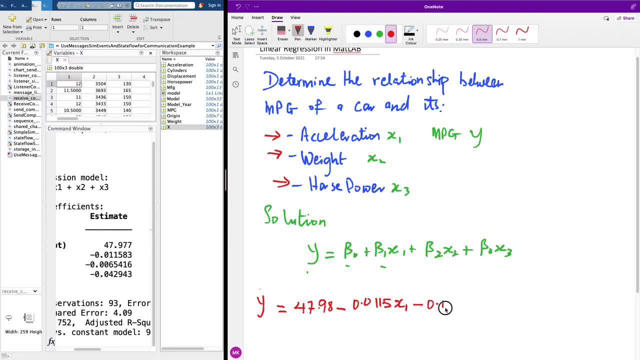 And again minus 0.0065 x2.. loss: minus, sorry, so this is also going to be minus here. so minus 0.043 x3. okay, so what i want you to do now? this is our equation here, so try to calculate the value of a of y given the values of x. 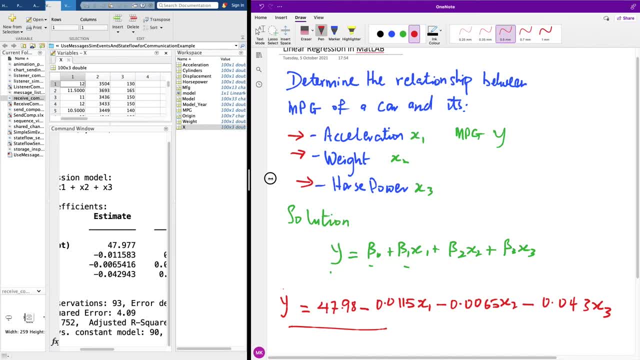 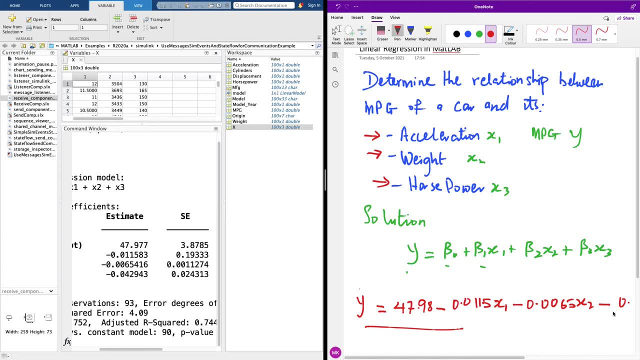 so basically, what i'm saying in fact is, if you look at this place, try to use the values you have here for x, substitute them here and determine the value of y, and then you go back to look, to look at the original data set, which is what we have here, and check the value of the mpg that corresponds. 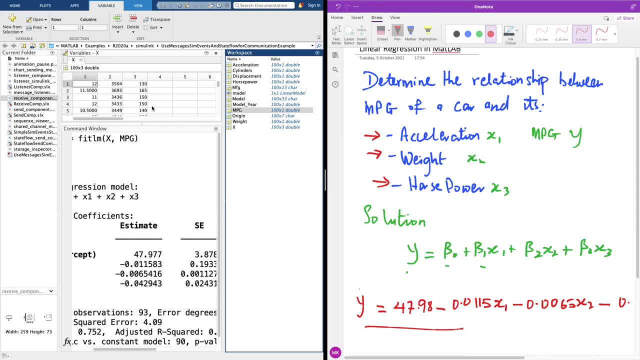 to the particular values you have. so i'd like to stop here. i'd like to thank you for viewing. i'm going to be creating nuggets like this for MATLAB in my channel, so please remember to subscribe to my channel and if you have any challenges, please do let me know. this is simple: multiple linear regression. 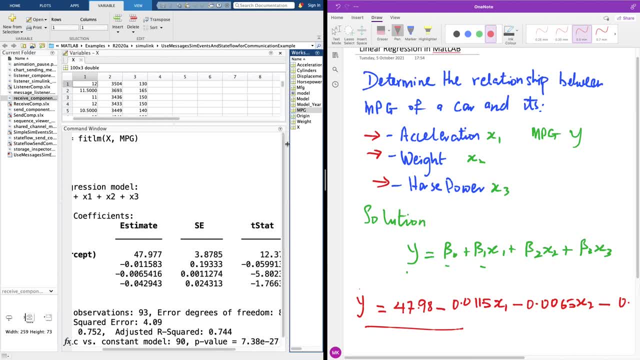 using MATLAB. so i remain kind to the genius and i'm always there for you.